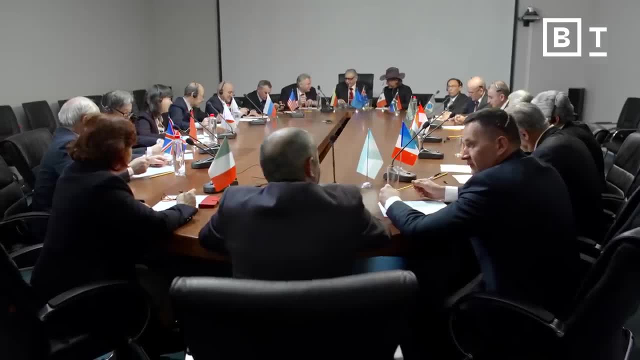 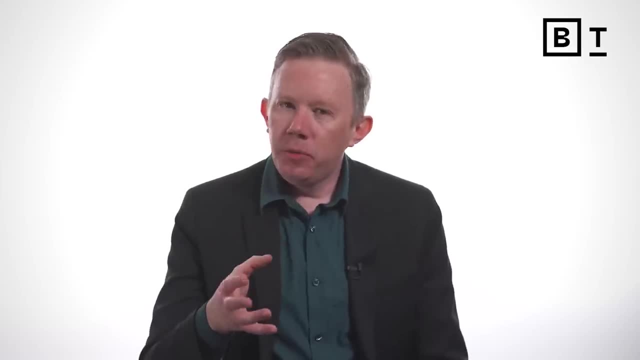 situations, including biology, international relations and even interpersonal relations like friendship and parenting and family relations. One of the things that game theory has really shown us through recent study has been interactions that we oftentimes think as zero-sum or competitive are not as competitive as they seem. 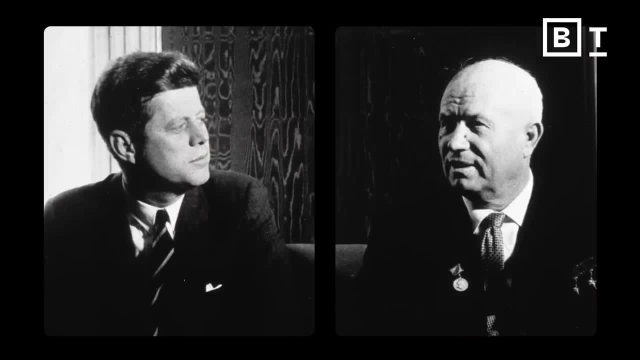 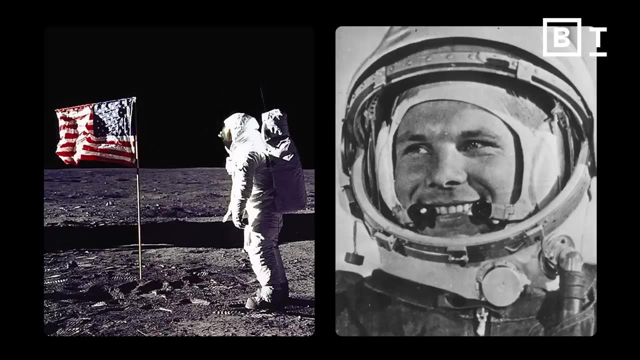 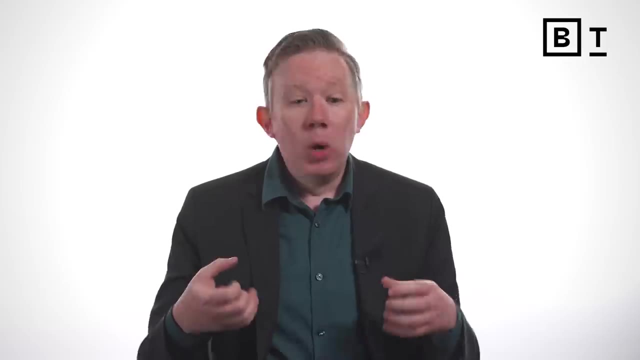 In situations like in the Cold War, which most people thought that's got to be a zero-sum game, if anything is, we discovered that actually there were opportunities for mutual cooperation. Arms reduction treaties are a great example. The US and the USSR figured out that if they could find a way to cooperate, they could 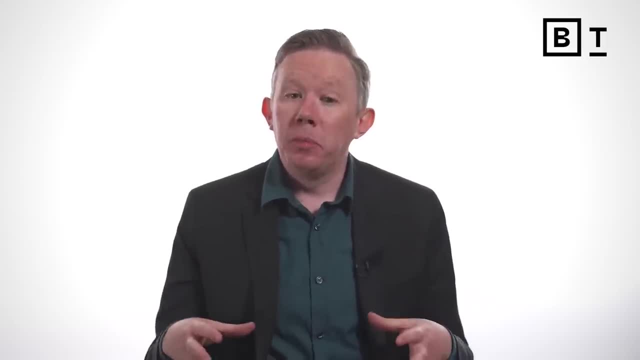 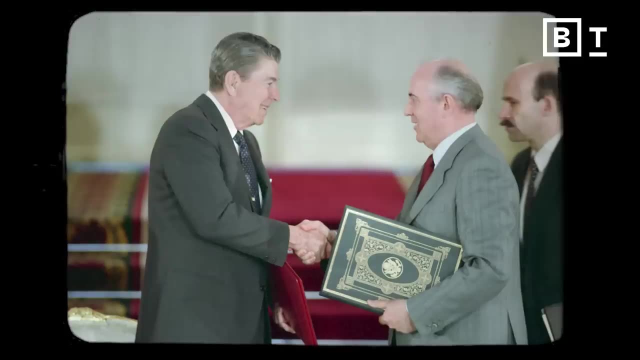 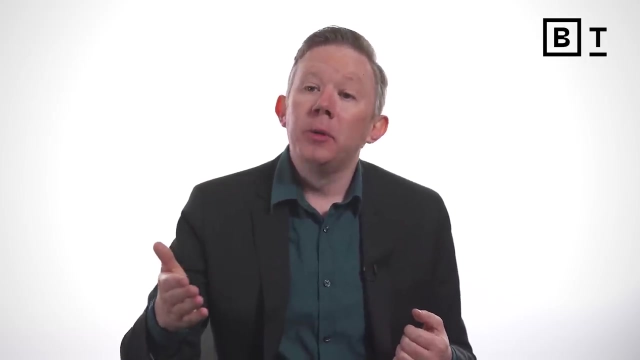 both save an enormous amount of money and effort by reducing the number of weapons that they have. Reagan and Gorbachev negotiated the START treaty with one another, and one of the big problems that they had is: How can you do this? How can you be sure that while you're eliminating nuclear weapons, your adversary is also eliminating? nuclear weapons. So rather than saying we're just going to get rid of some large percentage of our nuclear weapons and hope that the USSR would do so as well, they broke up the interaction into a bunch of little tiny ones. So the USSR would eliminate just a few nuclear weapons, then the US would eliminate just 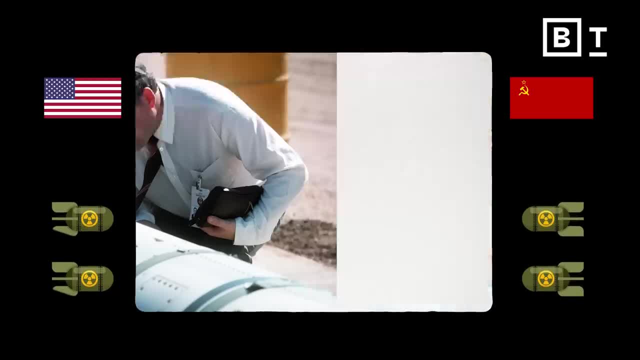 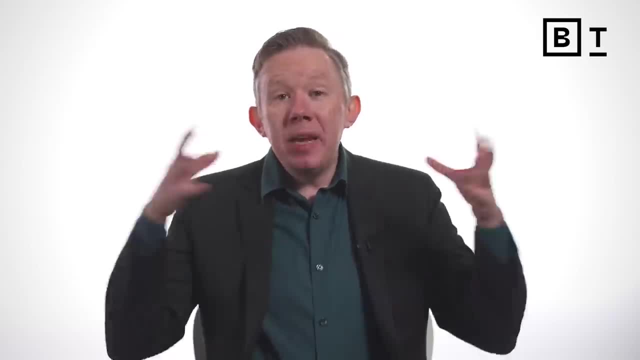 a few nuclear weapons, They would check, and then they would go on to the next stage, and then each would eliminate a few more and they'd go on to the next stage. This process of taking a big interaction and breaking it down into little, small parts. 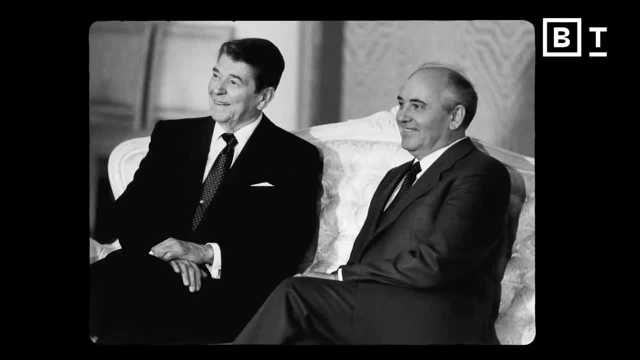 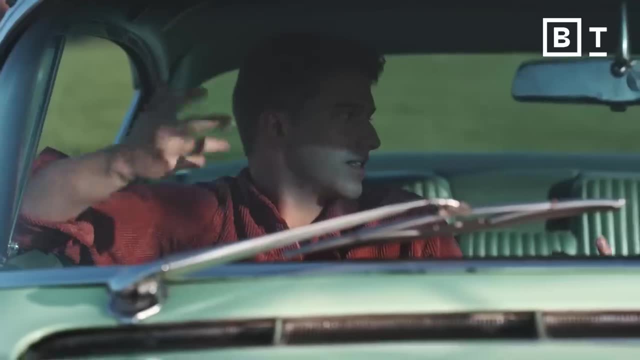 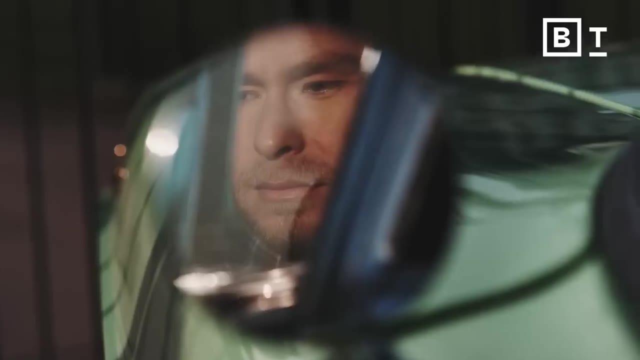 can change a bad social dilemma into a positive interaction. What I do in my personal life, and I think almost everyone can do in their personal life, is to try and think in this interaction, what outcome would be good for both parties And how can we achieve that outcome? 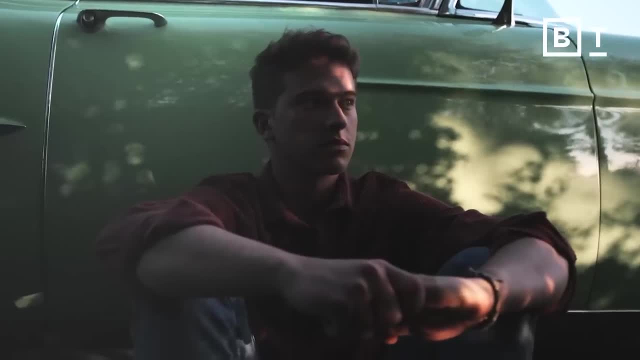 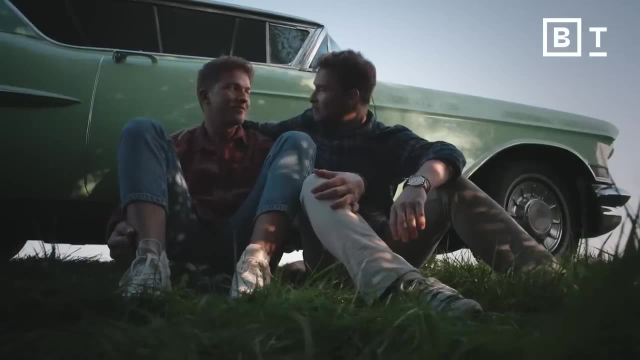 And by thinking about everything in that way, we oftentimes transform something that seems like a situation where they're happy, There has to be a winner and there has to be a loser into one where nobody feels like they've lost and everybody benefits. 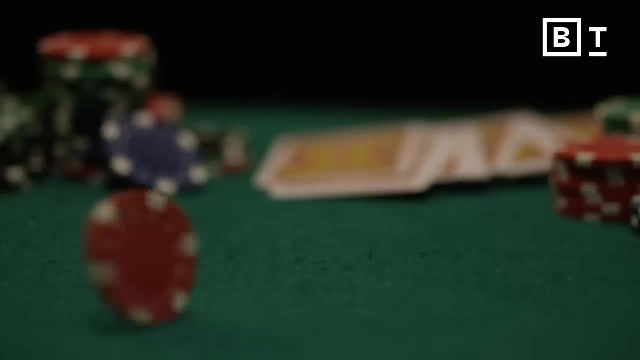 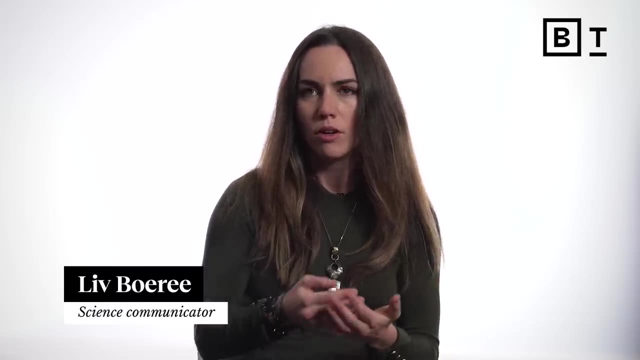 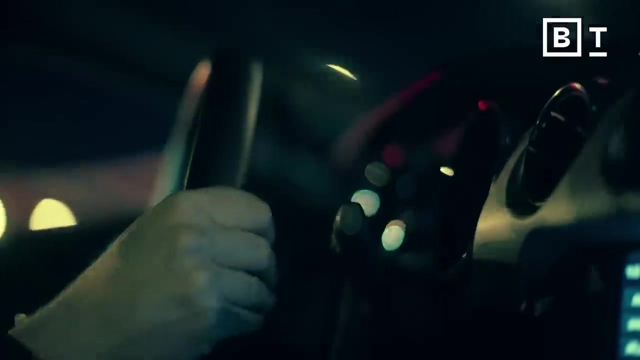 John von Neumann based Game Theory on a stripped-down version of poker. In any given poker situation, you're dealing with a lot of uncertainty and it's all about how to make the best decision in any given moment, and that's so integral to life. 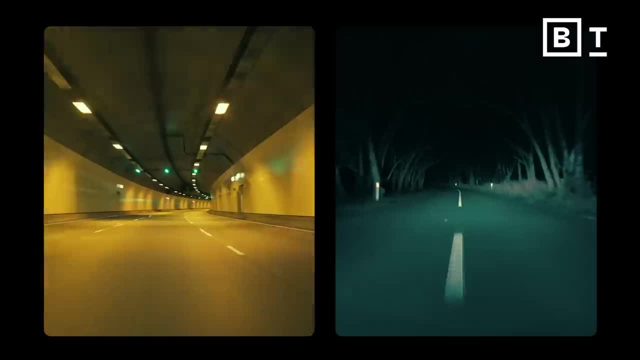 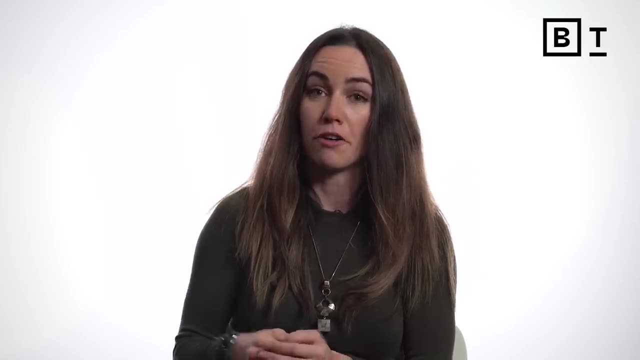 Everything we try to do, you know, should we take this route or that route? should I go here on vacation? It's all about dealing with uncertainties and probabilities of things happening, and poker is a very fun and easy way to teach someone how to do that. 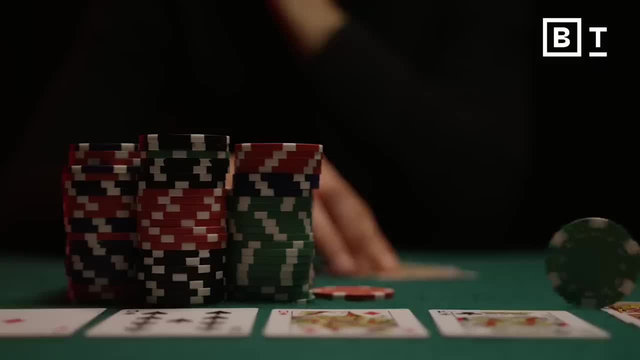 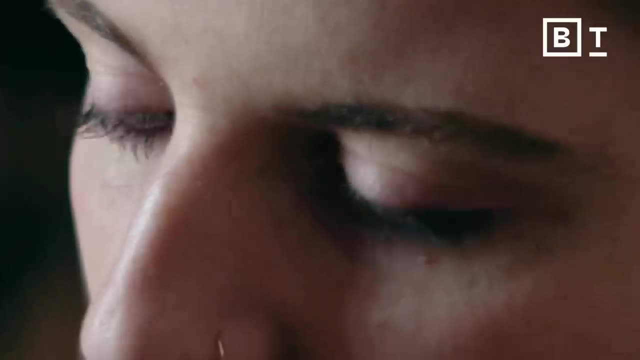 First rule of thumb is how to extract the most money or chips from your opponent when you have a strong hand and how to lose the minimum when you have a weak hand. You're never going to be 100% certain where you are. Are you beating them or do you have a worse hand? 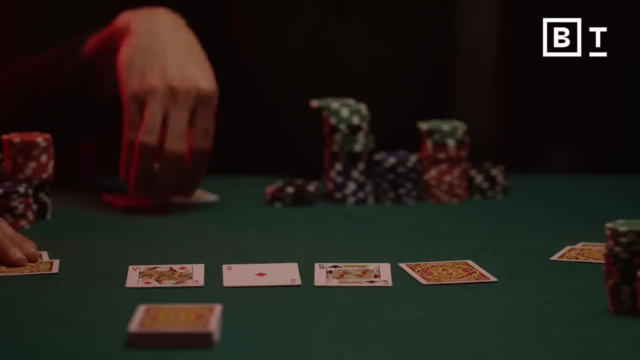 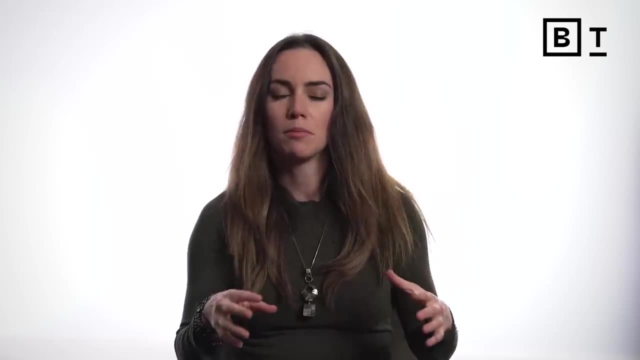 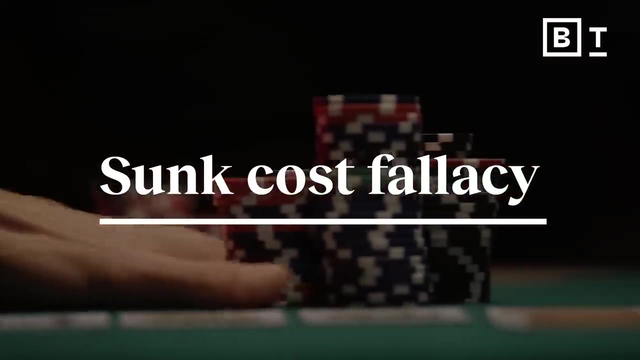 So you have to sort of construct a strategy that is It's mathematically optimal in each situation. The most damaging bias that can come up in poker- and I also think very often in life- is the sunk cost fallacy, where you'll have a lot of chips, perhaps almost all of your. 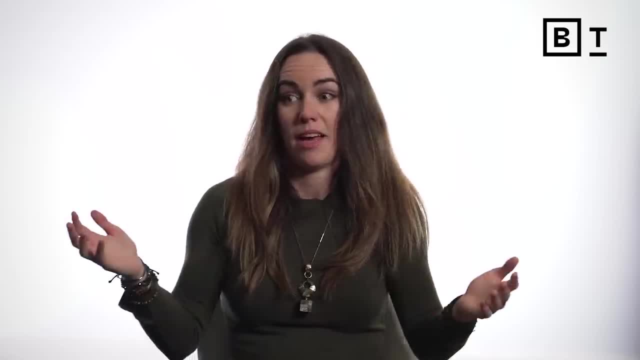 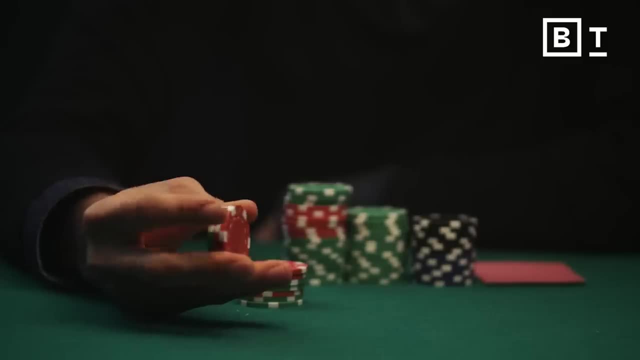 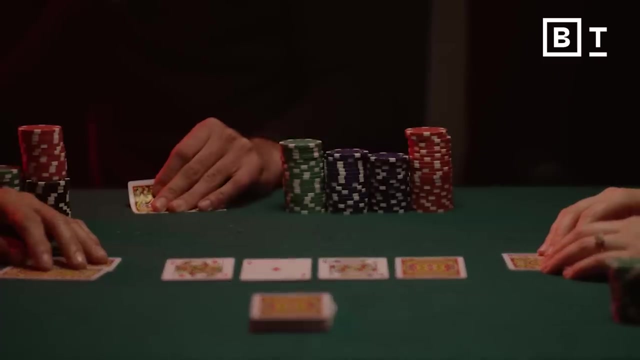 stack is in the middle and yet you are 85 to 90% confident that you have the worst hand. Putting another chip in the pot is probably not a good idea, but we'll often go to a game where we say to ourselves, well, I've gone this far, I've put this much in. I 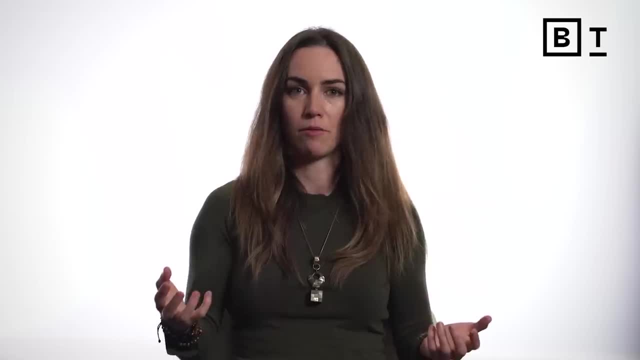 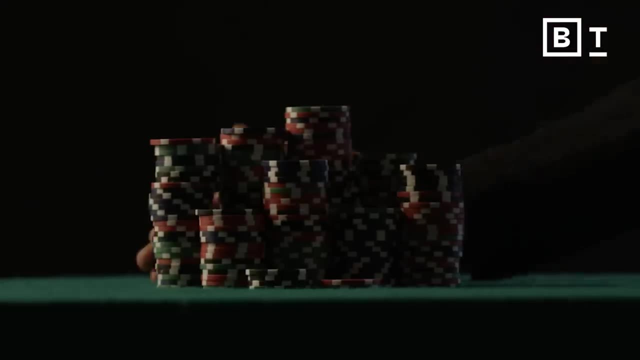 might as well see it through to the end. But if you have very strong information that actually, from this point onwards, putting more money in the pot is a bad idea, then you shouldn't. But we have this belief that well, I've put this much time in or this much effort. 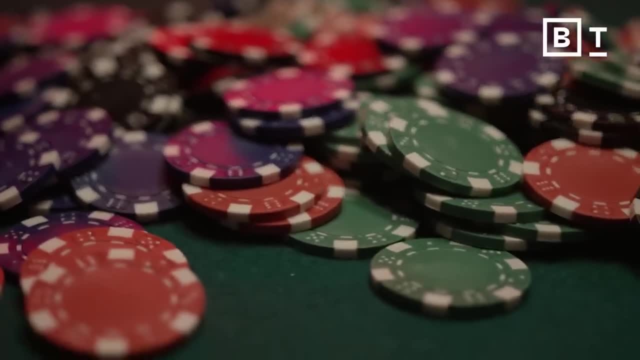 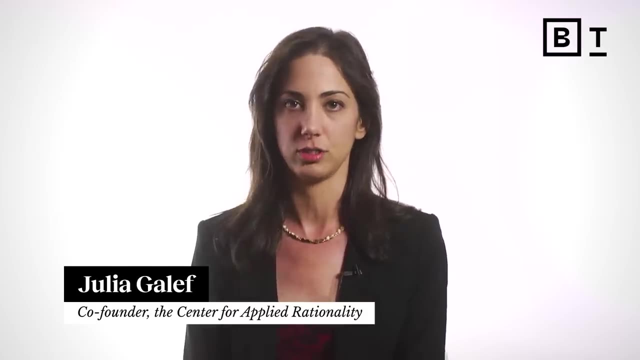 that we should continue on. That can be very, very costly. Once you start paying attention to the sunk cost fallacy, once it's on your radar, you'll probably notice at least a few things that you wish you were doing differently. Those might be small scale. 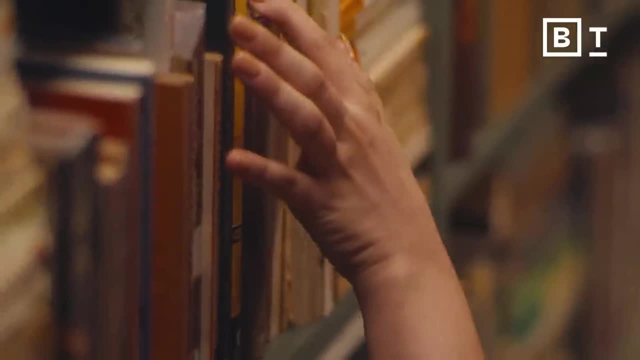 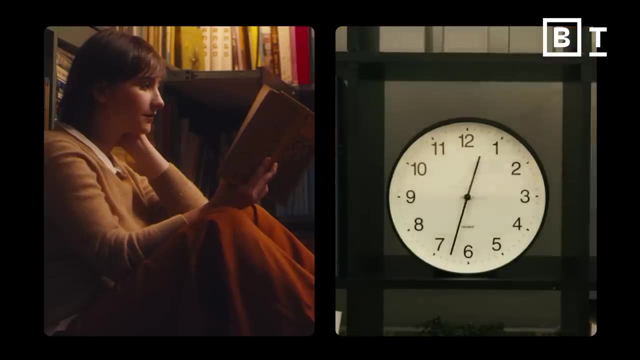 In my case, I'm now much more willing to abandon a book that I've realized I'm not enjoying and not getting any value out of, rather than trudging dutifully through the remainder of the book just because I've already come 100 pages. 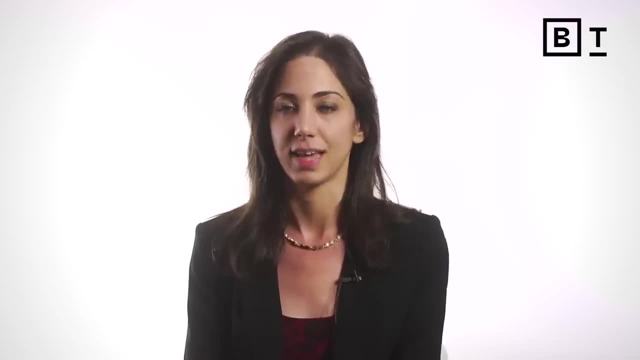 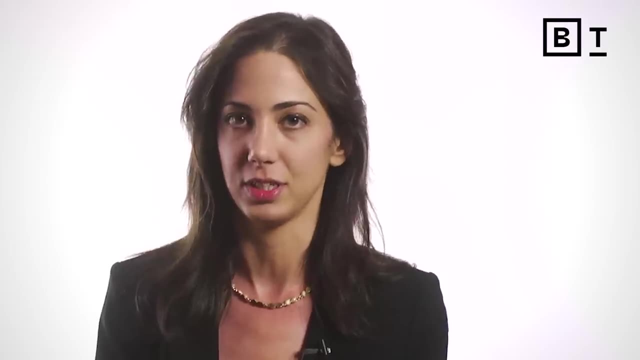 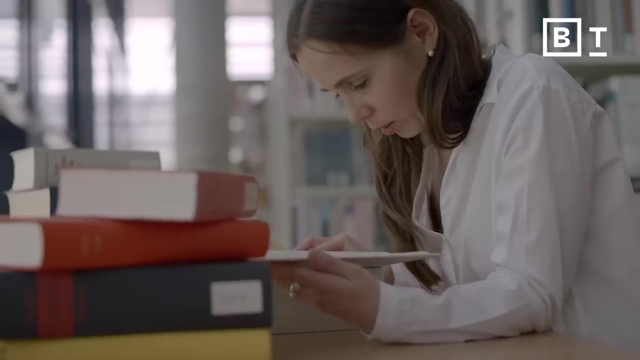 These changes might also be large scale. For example, I was in a PhD program and at a certain point realized with increasing certainty that I wasn't happy in this field and would probably be better off switching, and that the only reason that I had stuck with it as long as I had was because of my fear of confronting 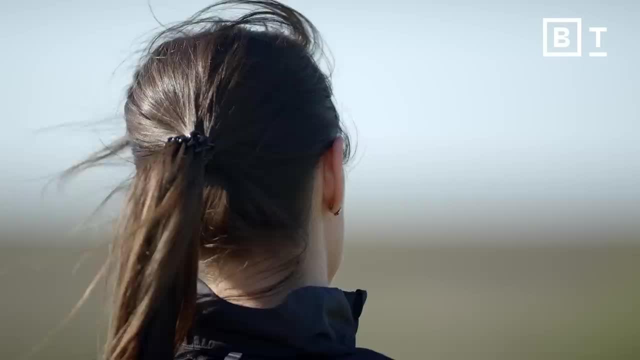 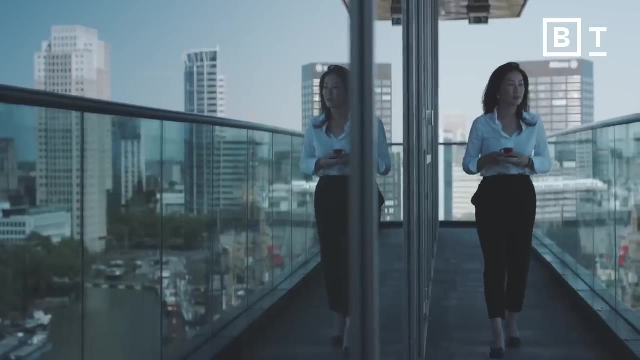 the sunk cost of four to five years that I'd spent preparing for and working in the PhD, And sometimes it really does take time to fully acknowledge to yourself that you don't have any good reason to stick with the job or PhD or project that you've been working. on so long because sunk costs are painful. But at least having the sunk cost fallacy on your radar means that you have the opportunity at least to continue To push past that and make the choice that instead will lead to the better outcomes for.